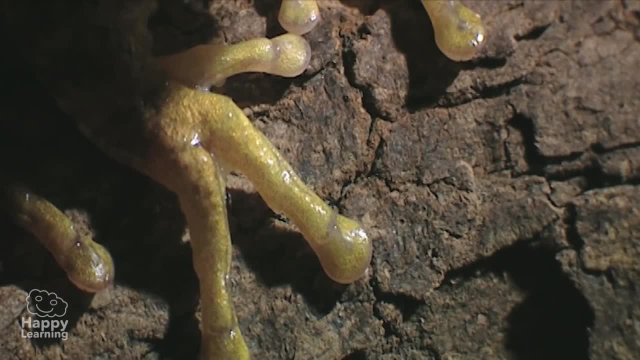 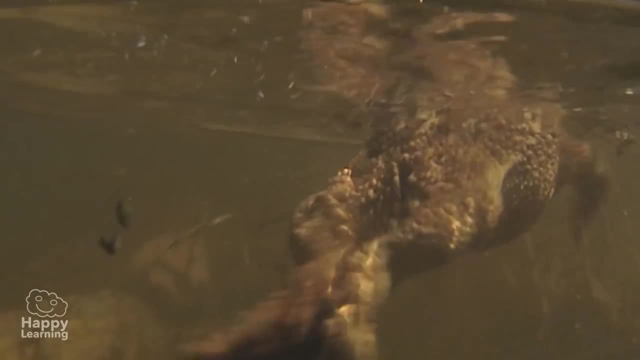 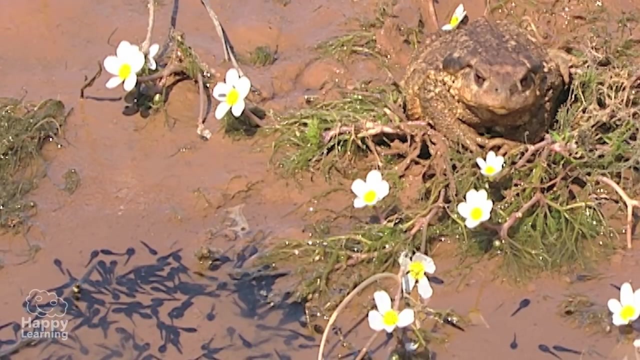 have four legs and a membrane between their toes that allows them to move much better in the water. Amphibians are aviparous, but they don't incubate their eggs. after laying them, They abandon them and don't care for their young, Not very good parents. huh. 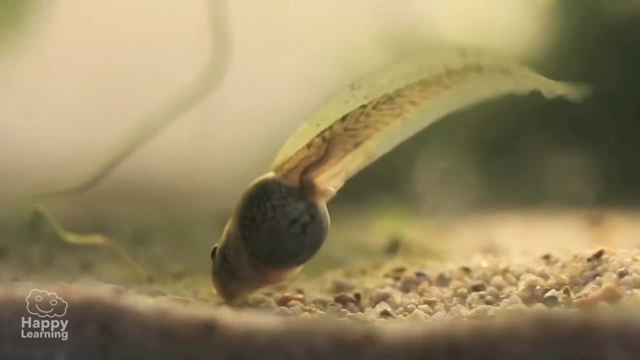 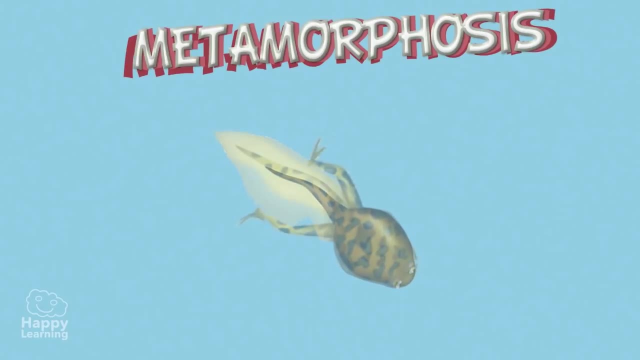 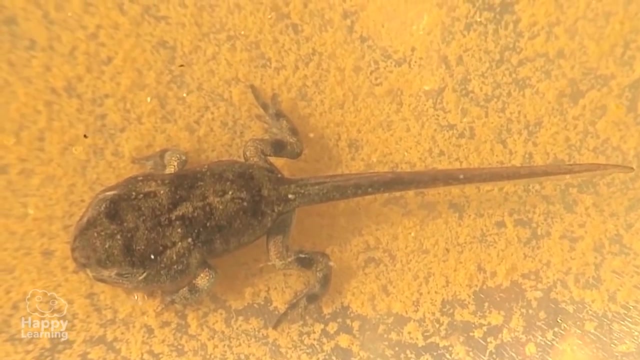 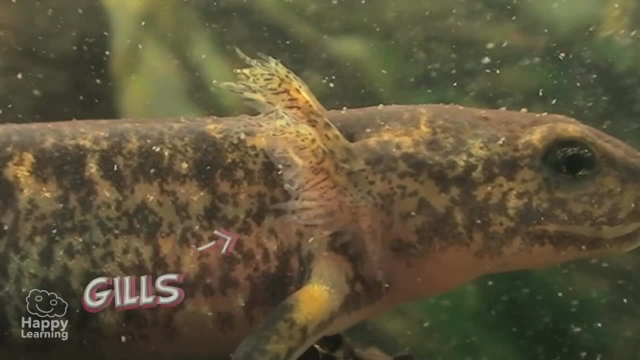 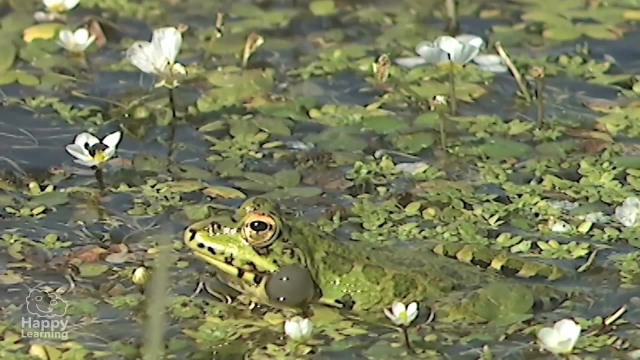 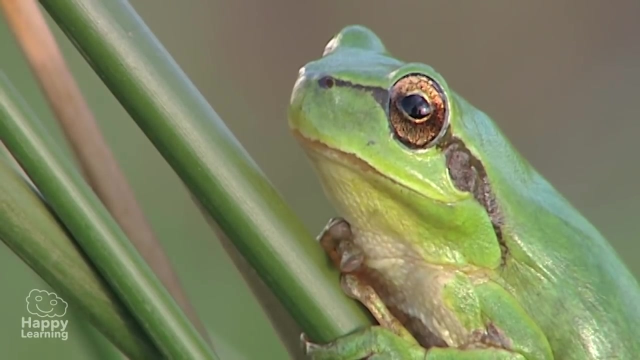 So they finally look like their parents. In the early stages of their lives, amphibians breathe through gills, But when they grow up and become adults, they breathe with their lungs. The problem is their lungs are very small and cannot get all the oxygen they need to live. 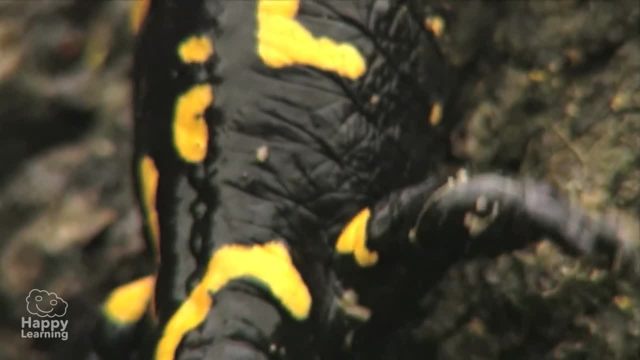 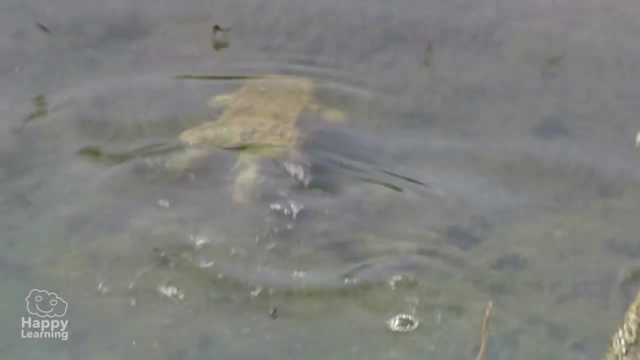 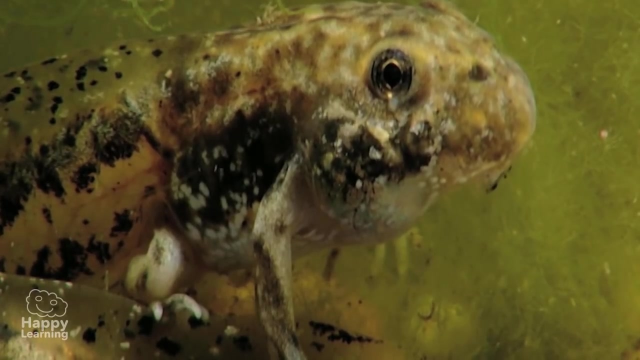 But nature is very clever and has solved this problem by allowing them to breathe and get the oxygen they need through their skin. That's why they need to be near water to keep their skin wet. In the early stages of their life, some amphibians are herbivores, But when they grow up, most 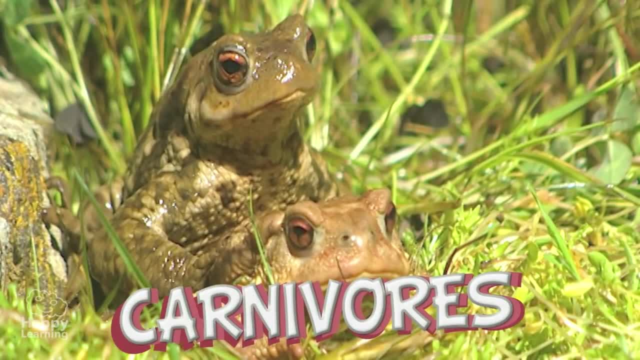 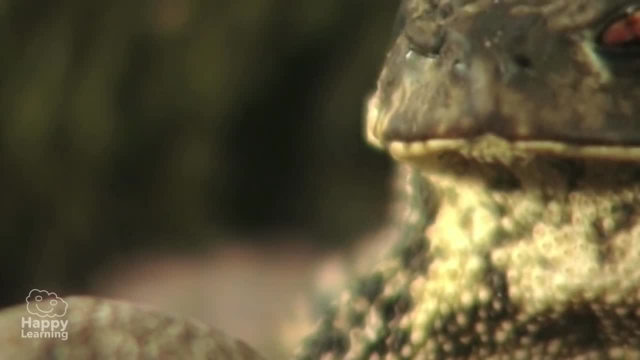 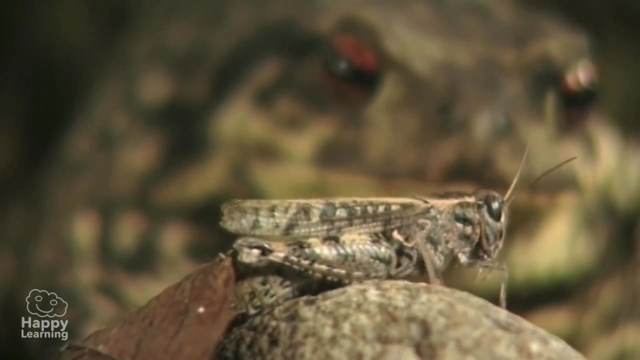 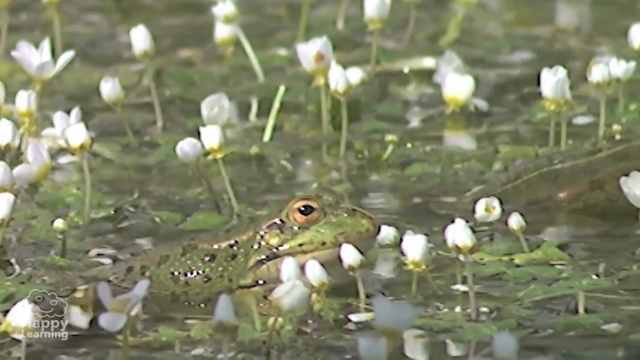 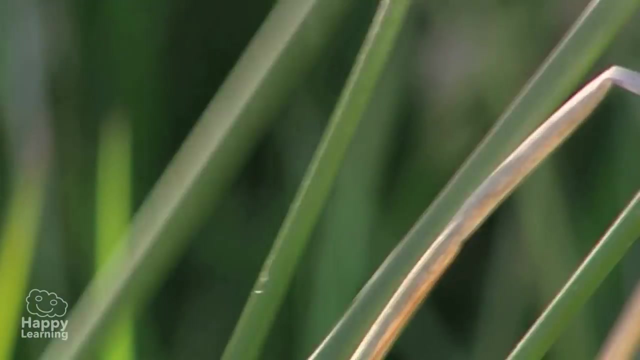 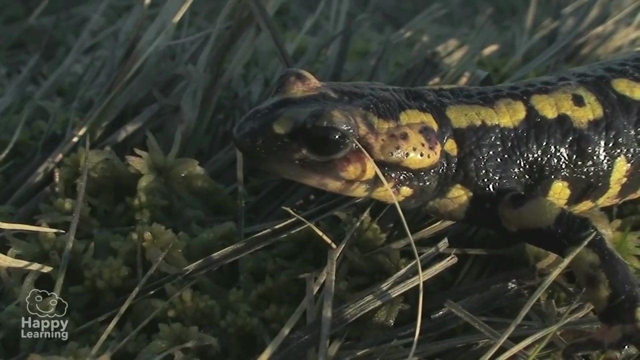 become carnivores, So they need to hunt. Some have a long, sticky tongue. They shoot out to capture prey. Aren't amphibians fascinating And also a bit strange? So let's remember the most important characteristics: Amphibians are vertebrates. They're oviparous.